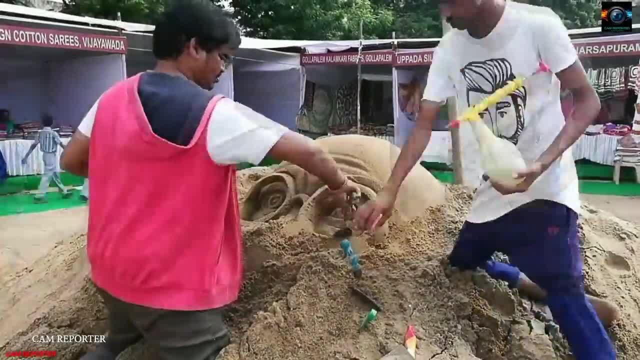 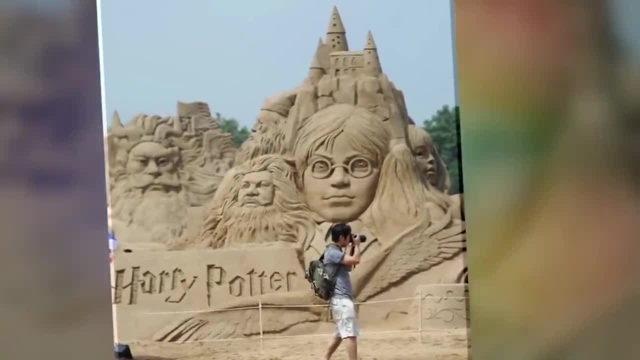 from the walls. It was built by an unknown artist as part of China's 2011 Changsha International Sandstorm Sculpture Art Festival. It's such a stunning piece of work that you won't forget this one, unless someone casts an Obliviate charm on you And you'll want to walk right up to it and shout. 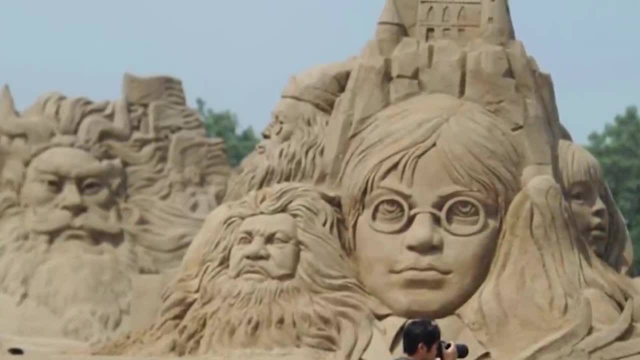 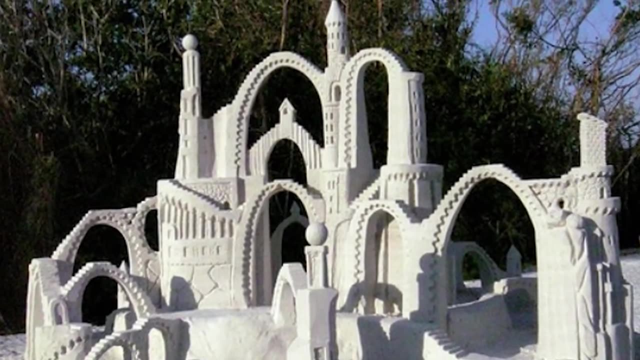 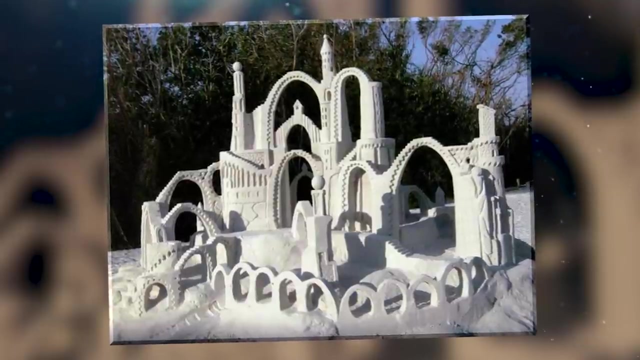 Alohomora, so you can walk right inside Number 14, White Sand Castle. There's not much I can say about this one that you can't see from taking a look at it. It's an incredibly detailed design that seems to almost defy gravity, Sculpted entirely from clean white sand. this creation, 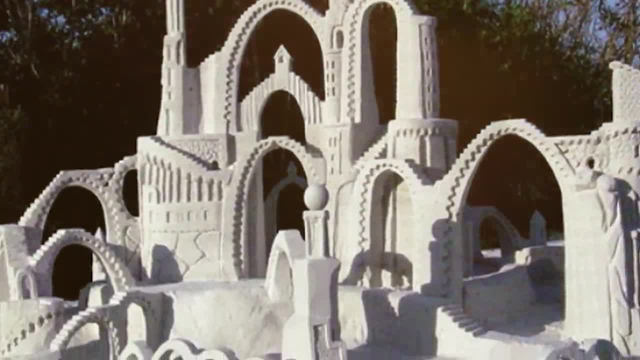 features a couple of dozen of sandcastles. It's a very unique design and it's a very important piece to take a look at, with these newdowns from ancient times Sculpturing on a fabric that resembles aging dead. 14th-century lightそれで, a major 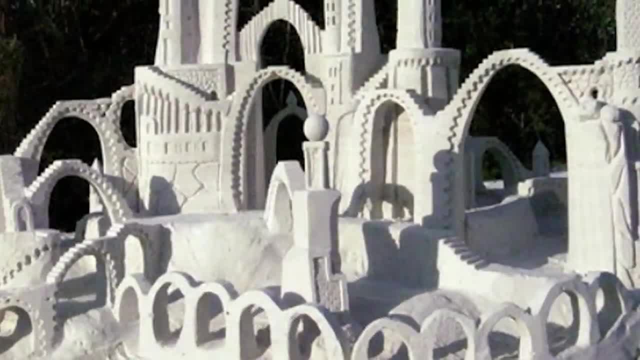 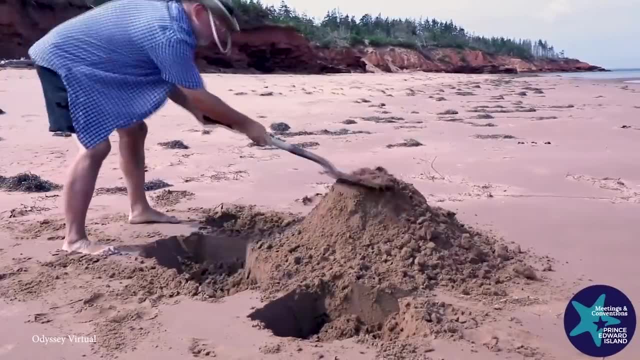 fixation on clouds of did weaneges, walls and arches. Getting to the frame of the castle чи, a small arch goes really井and some intricate windows carved into the castle's walls. It looks like a cross between King's Landing and an M C Escher painting. Unfortunately, 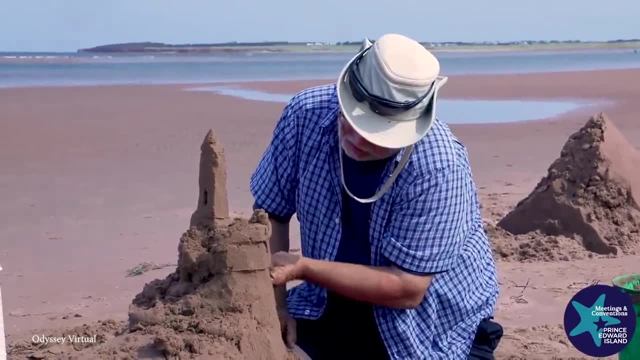 not too much is known about who created this beauty or what was made for, but that doesn't mean we can't appreciate that. beautyauraj gaben. One of the interesting things about sandcastles builds is that the artists generally aren't doing it for fame or glory. They're doing it instead because they love what they do. 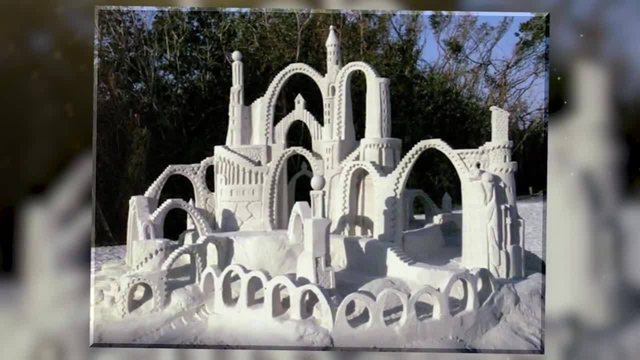 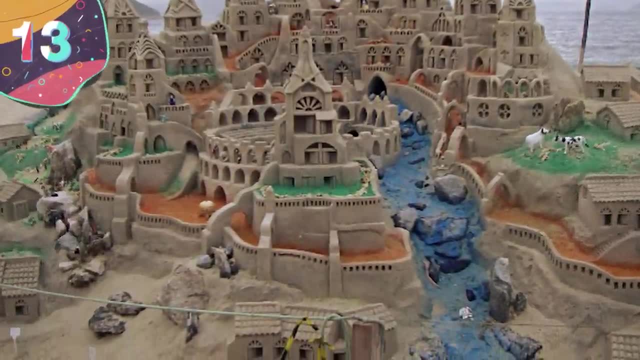 or would like to ticket that that stop hugeness. it's configur category that webelive white sand and it looks great in the shadows too. Number 13,: Colorful Sandcastle. This is another one of those sandcastles where not a huge amount is known about who made. 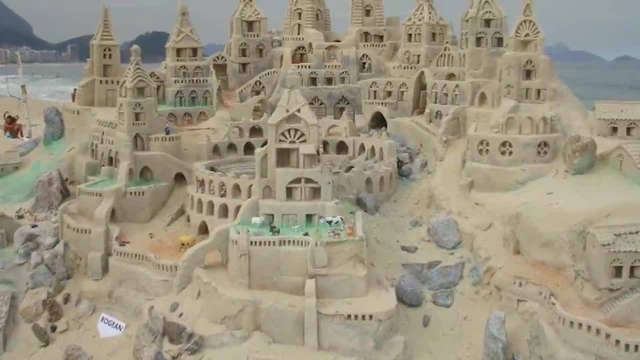 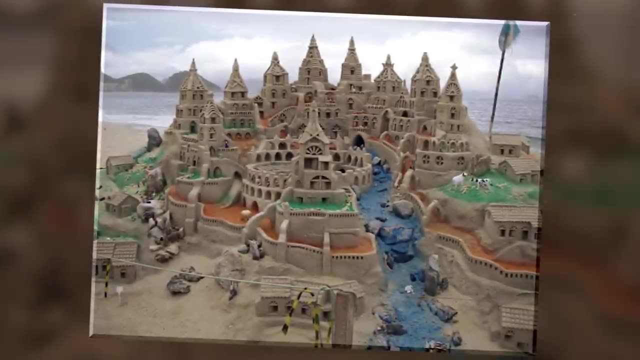 it or where they made it. I guess we can have a pretty good guess at why they made it, though. It's because it looks freaking awesome, As you can see from just taking a look at it. the most impressive thing about this one is that it uses a range of different colors. 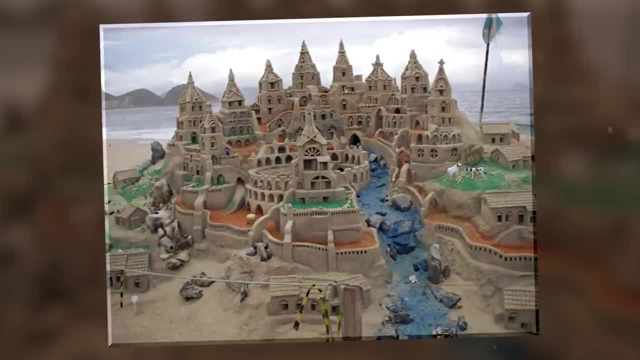 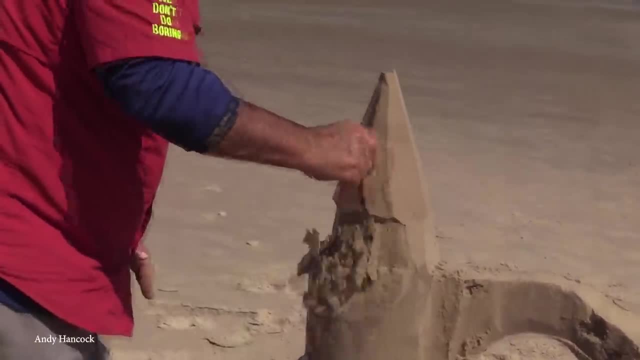 I'm not sure how the creator pulled this off, but we're guessing that it's similar to the way that colored glass is made. The sandcastles are different. For a start, they're much less durable, and it's not as though glass itself is known. 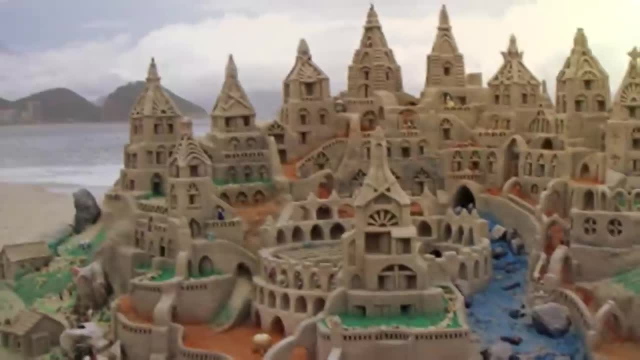 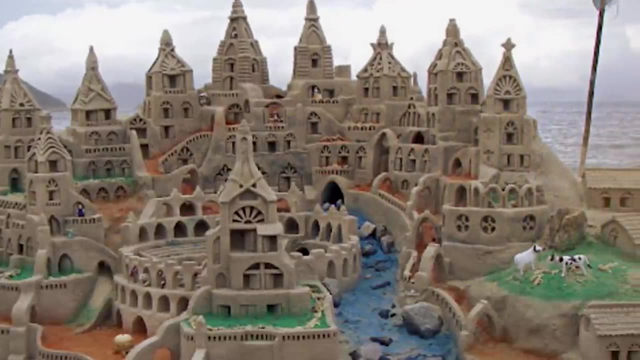 for being able to take a beating. This colorful sandcastle looks as beautiful as any stained glass window, but it would also wash away into nothing with a heavy rain or a few waves from the sea. Still, I think it's beautiful enough that it was worth the effort, and it's more than 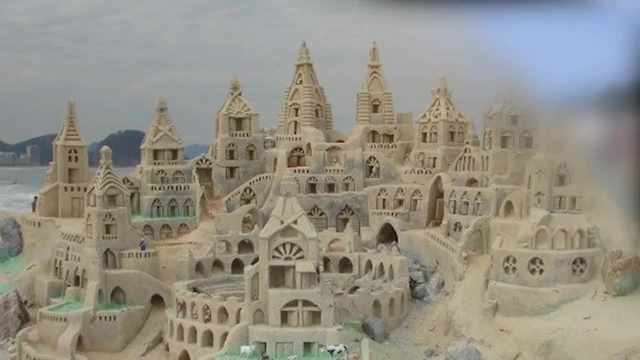 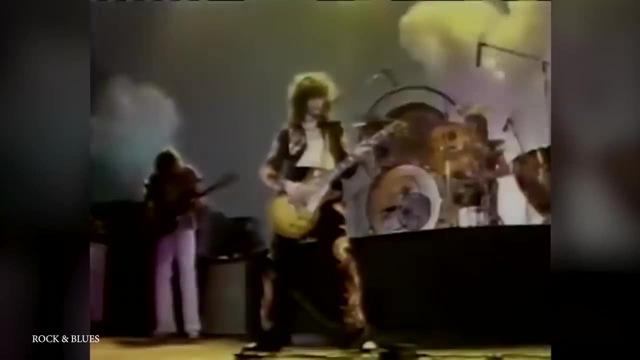 deserving of a spot on this list. Number 12,: Stairway to Heaven. There's a lady who's sure all that is What glitters is gold and she's buying a stairway to heaven. Weirdly, this is the second video that we've made recently that contains a reference to 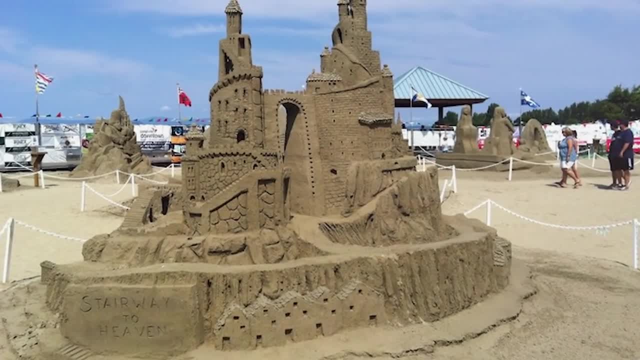 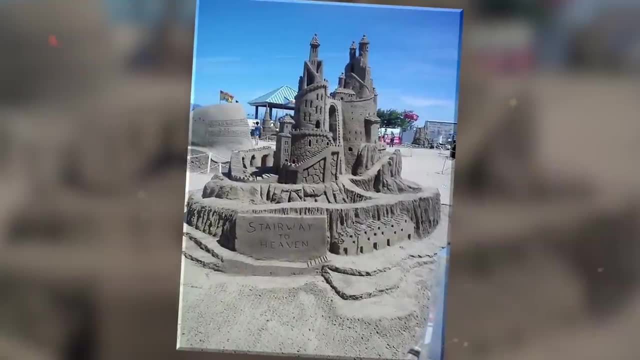 the iconic Led Zeppelin song. The last one was a stunning sculpture, and you could argue that this is the same, but that it just uses a different raw material. True, this sandcastle doesn't quite stretch all of the way up to the heavens, but it's. 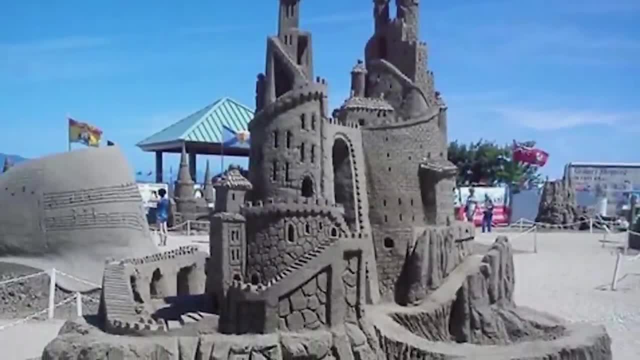 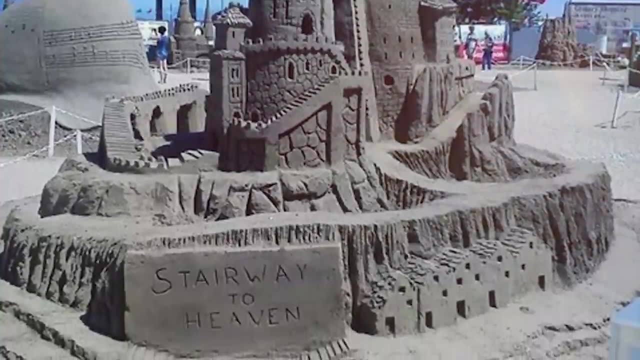 definitely off to a good start. It's one of the taller sandcastles on this list and it features a bunch of impressive design features and walkways. It puts us in mind of the Battle of Helm's Deep and the Lord of the Rings, The Two Towers. 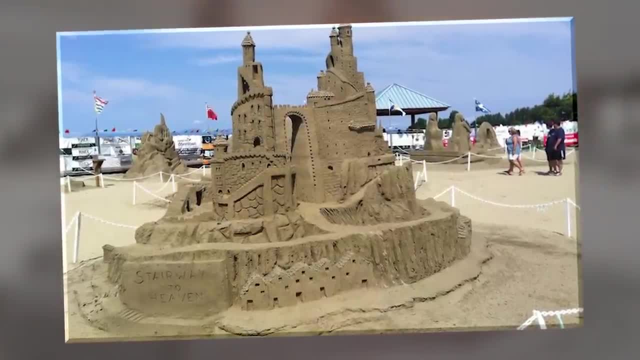 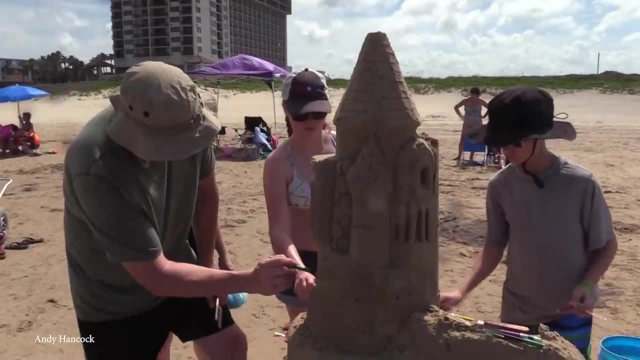 I'm not quite sure where this one was made, but we're guessing from the background of the photo that it was at some sort of competition. Either that or today's kids are getting insanely good at building sandcastles, because the ones we can see behind it aren't bad either. 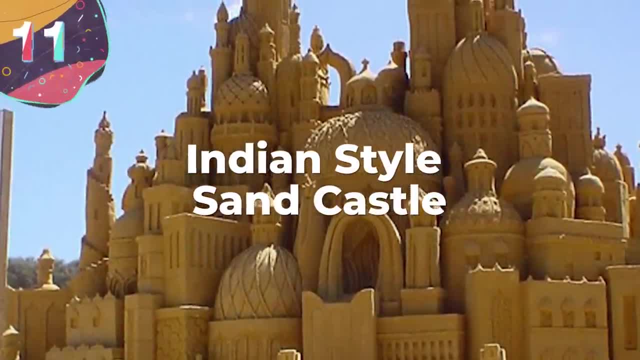 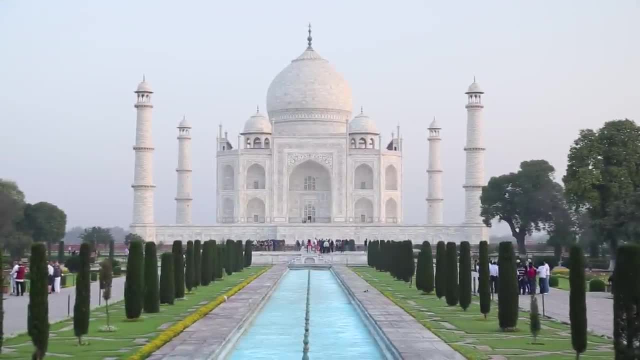 Number 11, Indian Style Sandcastle. To tell you the truth, I wasn't quite sure what to call this one, but there's something about the way it's built that reminds me of the Taj Mahal. I'll talk about that a little more later. 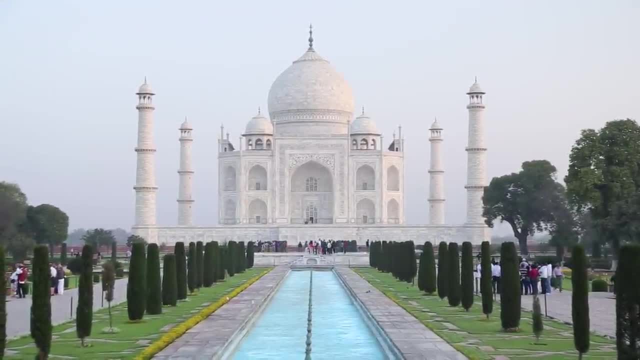 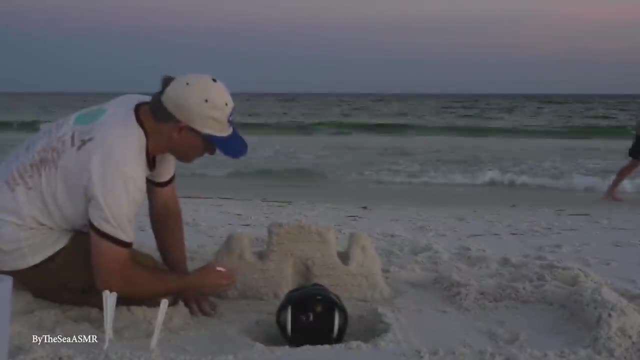 I'll be back with a new video soon, But perhaps it makes more sense to call this one Indian-inspired, because it actually uses architectural elements from all over the world. Talking about architecture when we're talking about sandcastles seems a little bit strange. 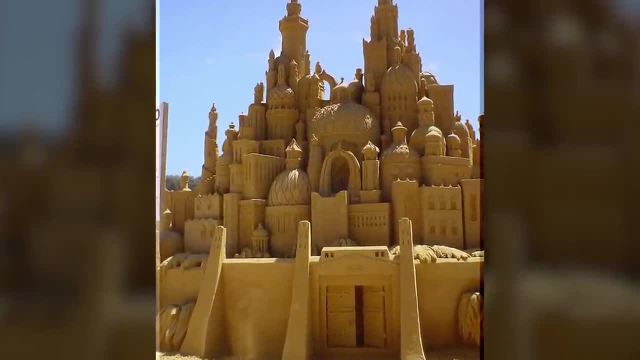 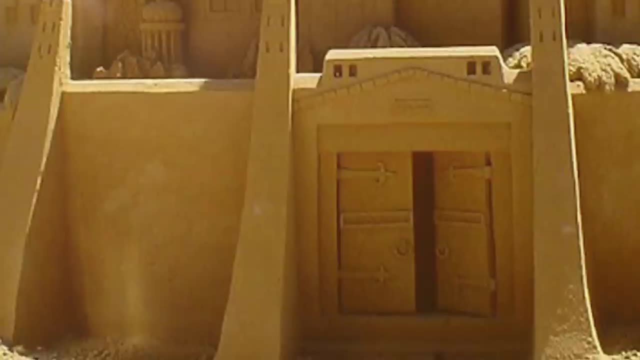 but one look at this photo is all it takes to see that, in this case at least, it is justified. I love the domes and the details on the windows, and I also like the way that the front door is half open, as though it's just waiting for you to walk inside. 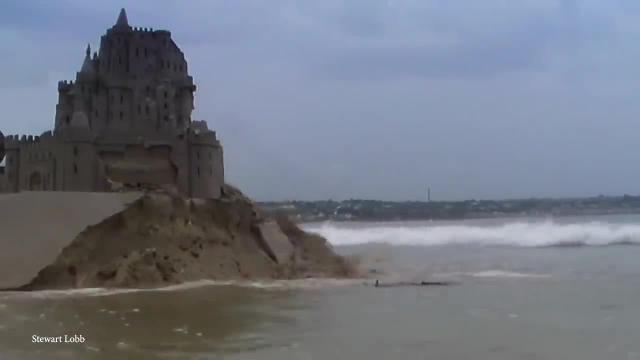 The only problem is that if you tried to do that, you'd quit. You'd quickly destroy the place, and it's far too beautiful for that. Instead, I hope this sandcastle was left to stand for as long as it could, although I 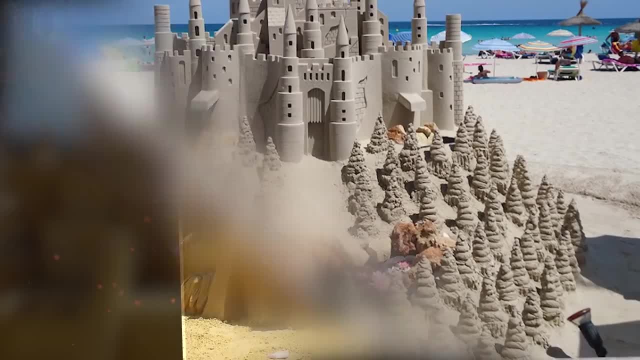 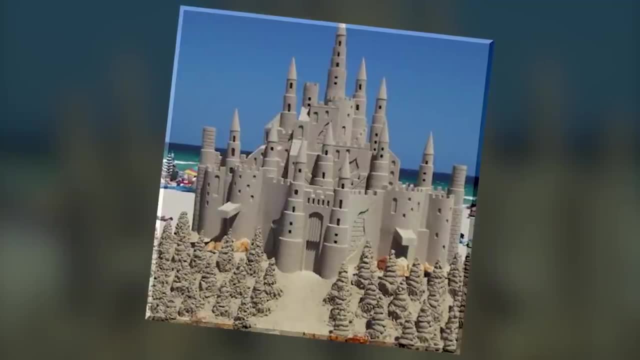 doubt that it's still there now. Number 10, Drip Sandcastle. This sandcastle would be worth a mention for the castle alone, which is a pretty impressive creation that looks out of place, set to the backdrop of a calm blue sea and sunbathers. 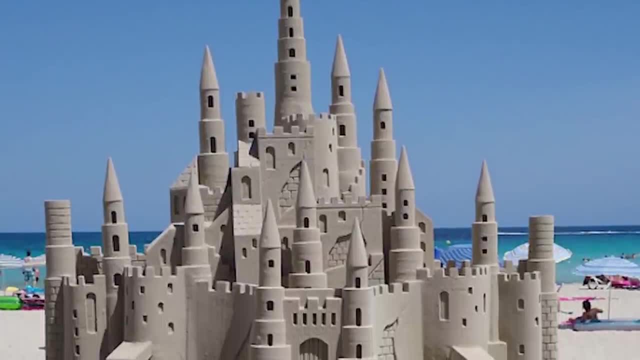 with their towels and parasols, But it's the drip-style enhancements on the hill of sand that put it in place. The sandcastle itself is a pretty impressive creation that looks out of place, set to the backdrop of a calm blue sea and sunbathers with their towels and parasols, But it's the drip-style enhancements on the hill of sand that puts it in place. 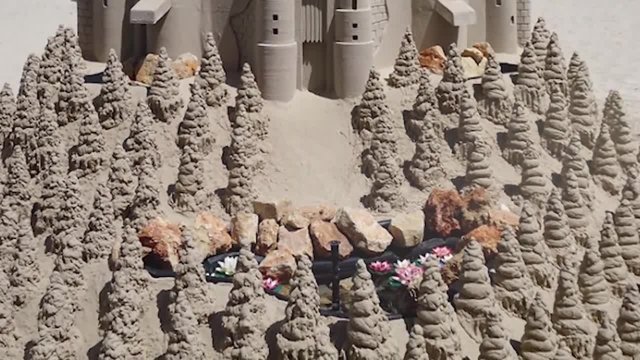 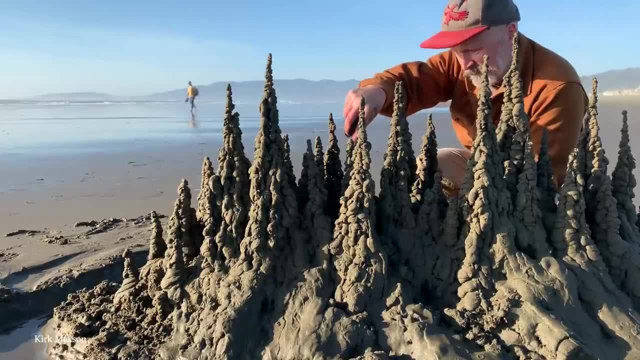 Thelive sandcastle was particularly caught in my eye, especially because I'm not quite sure how they even made them. I guess they were assembled separately and then moved once they were ready. Like some of the others we've taken a look at today, I was impressed with the attention. 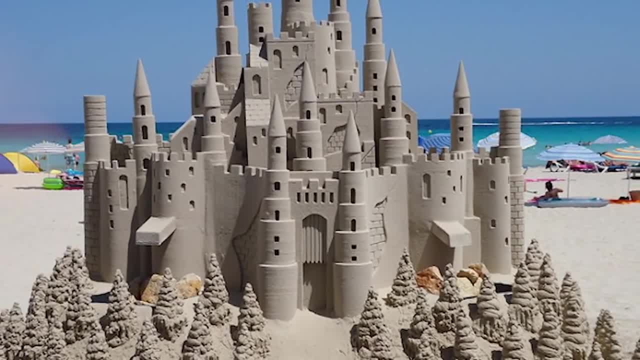 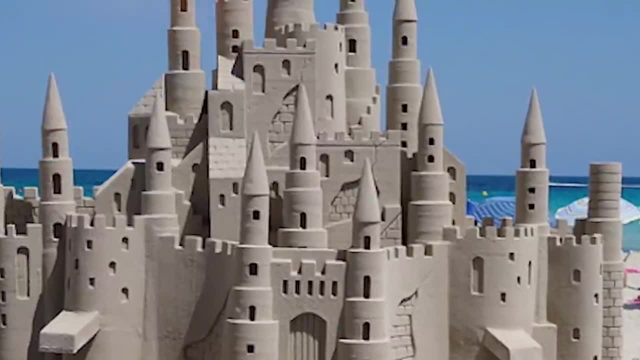 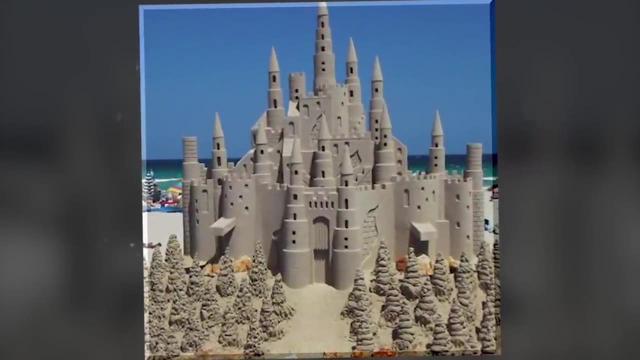 to detail, especially when it comes to the windows, which are surprisingly difficult to do. Both spires at the top are particularly impressive because they manage to hold their structure while simultaneously having windows carved into the sand. Overall, this sandcastle shows a remarkable amount of creativity and dedication. 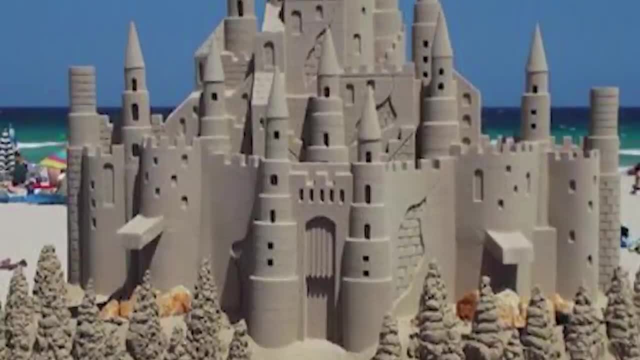 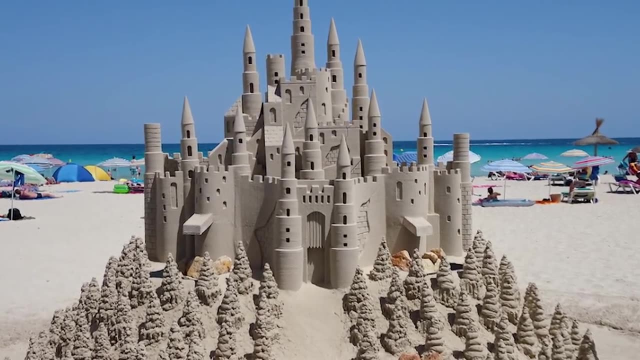 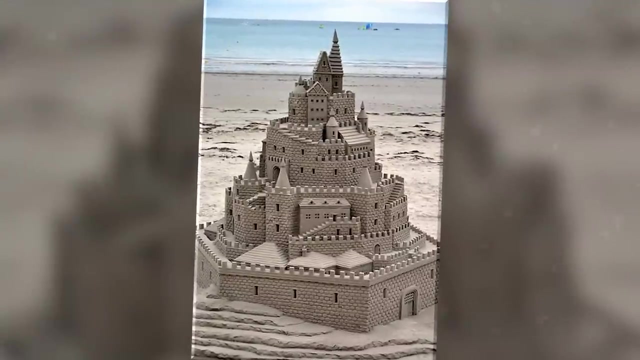 dedication to the craft, and I'd argue that it looks even cooler because it's not competing with any other castles in the background, as you often see when they're built as part of competitions. Number 9. Castle Sandcastle. This sandcastle is perhaps the one on this list that looks the most like an actual castle. 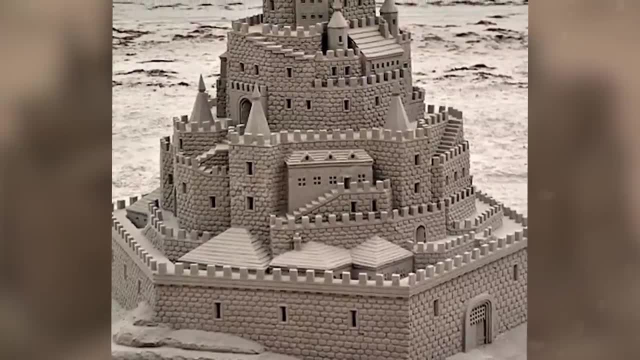 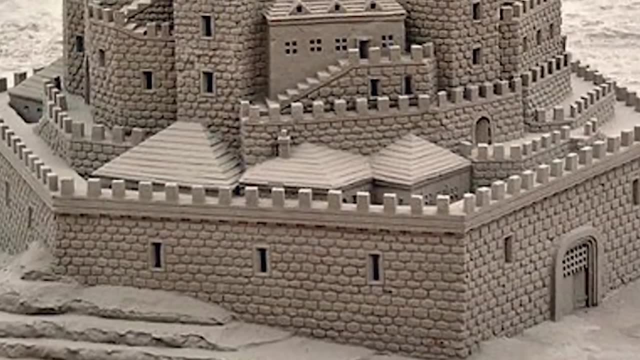 One reason for that is the design itself, which typifies the popular castle design, in which concentric walls serve to provide fortresses within a fortress. The other way is that the way the builder has spent so much time on the brickwork, which I guess took about as long as 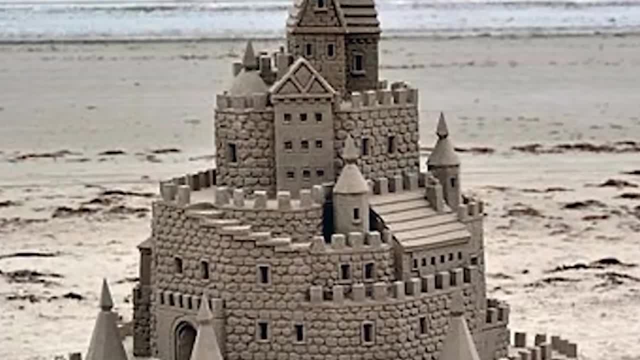 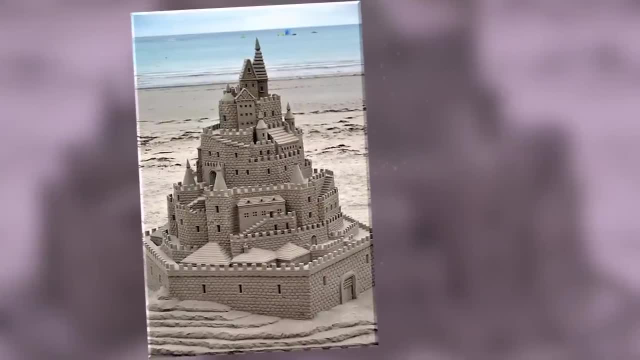 the castle build itself. Whether seen from close up or far away, it adds a layer of realism to the build that makes it look like the real deal. I also like the way that the creator of this castle has done such a good job of smoothing out the sand, which is in stark contrast to how rough 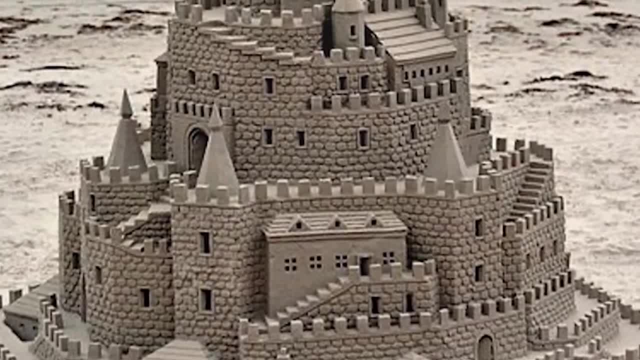 and lumpy it looks on the backdrop. There's also something about this one that makes it look cozy, or at least as cozy as a sandcastle can ever look. All in all, this is probably one of the best castles in the world. 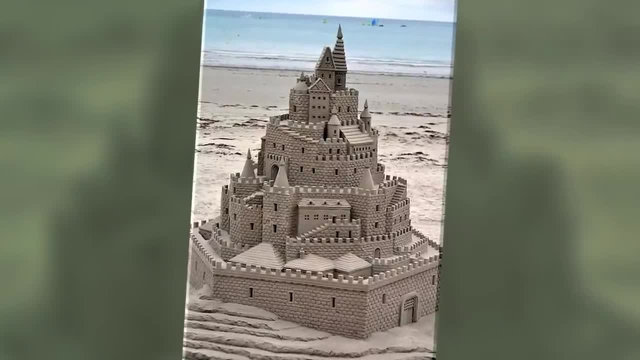 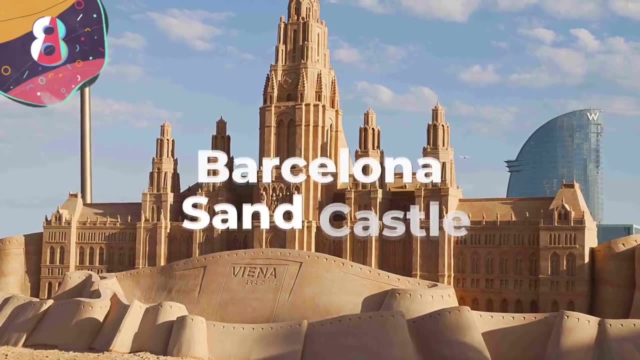 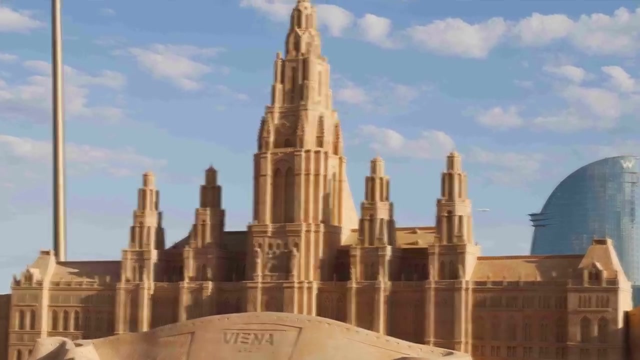 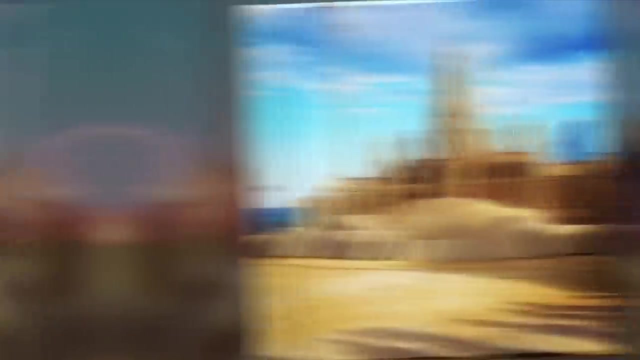 8. Barcelona Sandcastle. I've called this one the Barcelona Sandcastle because it's one of the few builds where we know exactly where it was built, although I don't know who built it or why. Based on the way it looks, though, you might have been able to guess the country of origin and at the very 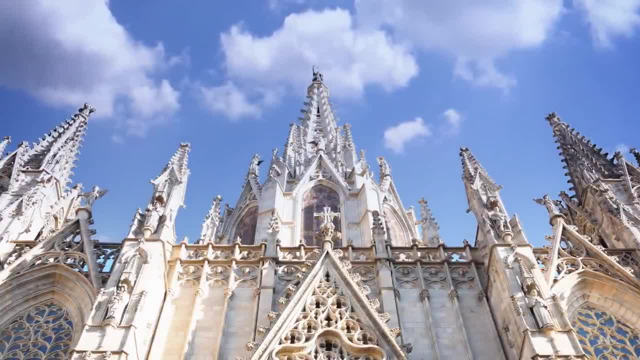 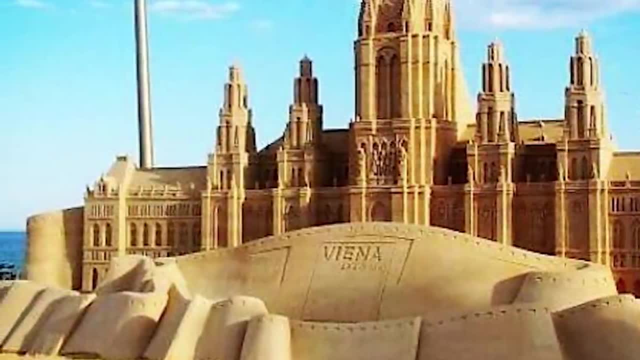 least you'd be able to tell that it was Spanish inspired. There's also something religious about this one feeling like a huge cathedral as opposed to a true castle. Yet again, it's the attention to detail that really shines here. Some of those spires look as though they 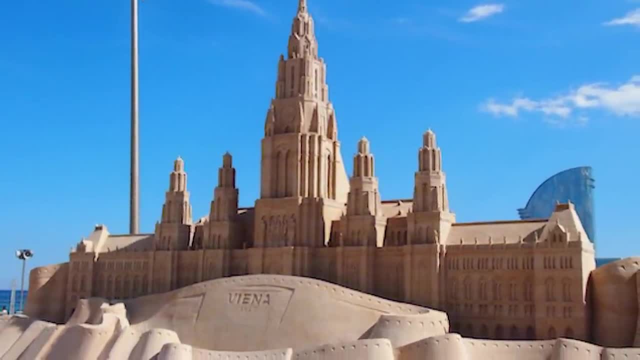 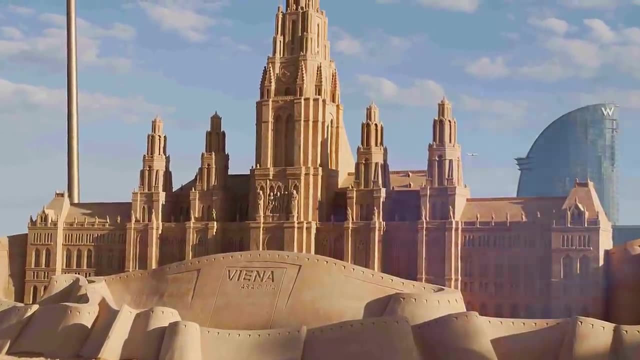 ought to collapse under the weight of gravity, and it's almost got me wondering whether the artist used something more adhesive than water to hold the thing together. But even in the unlikely event that they used superglue, we still think it's more than worthy of a place on this list. 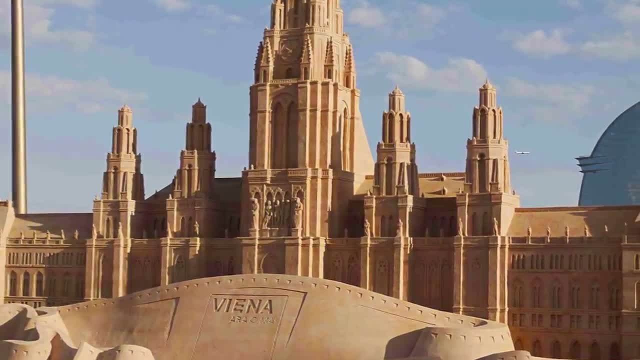 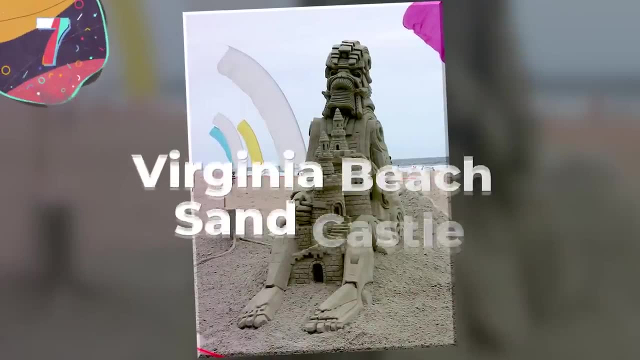 There's no way for us to know enough about the construction of these castles to do anything other than to build them. So let's take a look. 7. Virginia Beach Sandcastle. This incredible sandcastle was built on Virginia Beach in the United States. 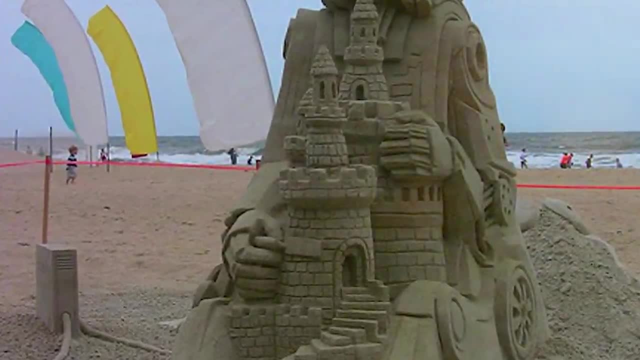 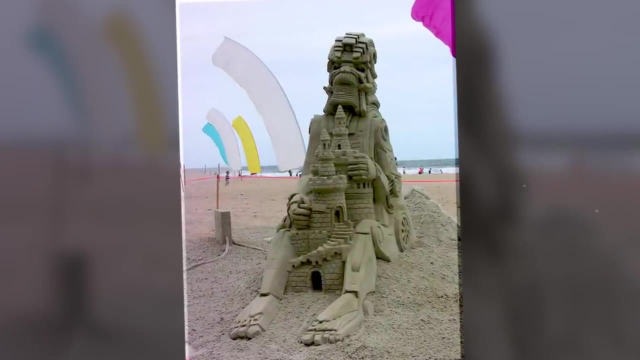 and while the castle itself is pretty cool, it's the sculpture that's built around it that really catches the eye, Depicting what I can only guess is some sort of samurai. the impressive thing here is that the castle pales almost into insignificance beside the warrior that's holding it in his lap. 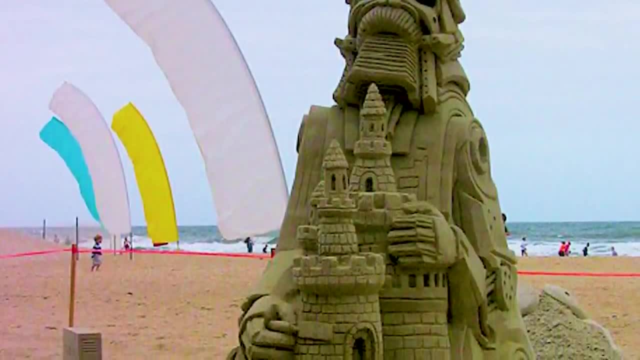 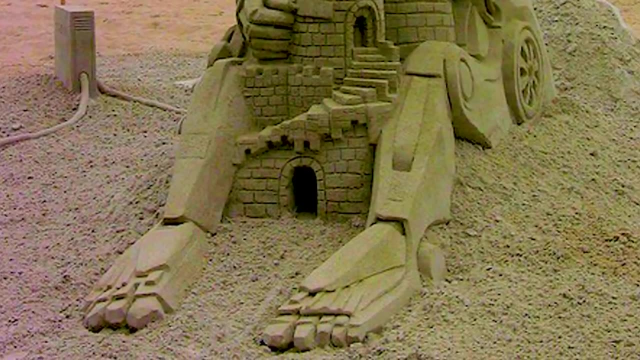 This is one of those castles where, if you were to build a castle, you'd have to build a castle where, if you attacked it, the boiling tar and the flying arrows would be the least of your worries. I really like the guy's hands and feet, because it's notoriously difficult for artists to replicate. 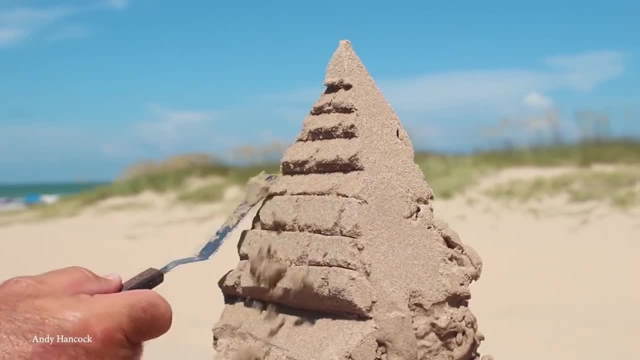 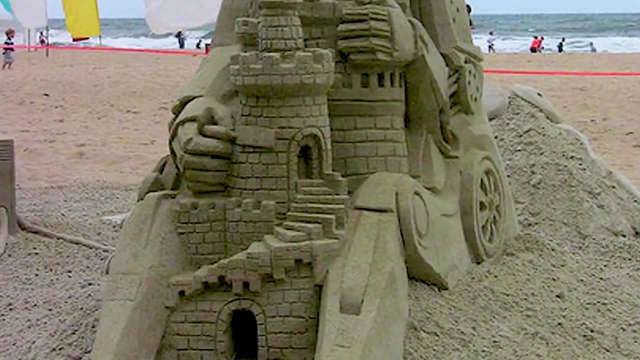 human limbs and appendages. I can only imagine that it's even more difficult to do it with sand, even granted that they're a little stylized. I'm not quite sure what that wheel is for, though. You'll also notice that the skies in the background don't look particularly appealing. 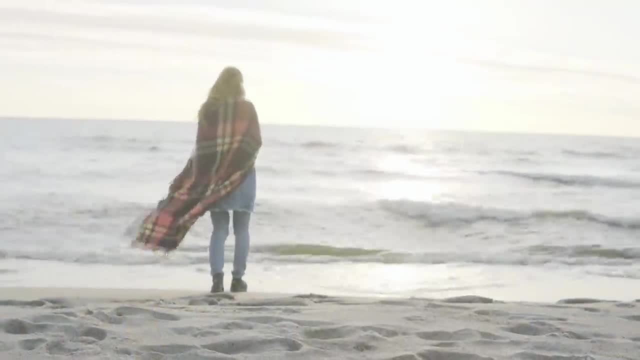 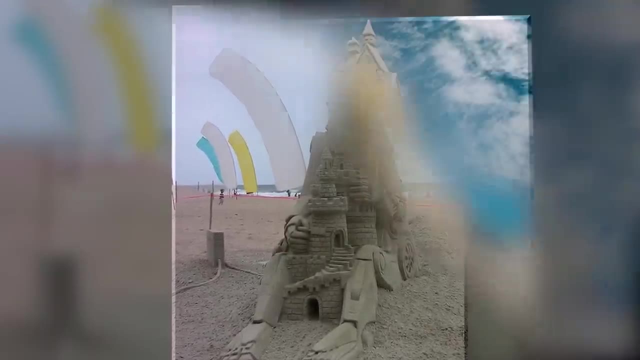 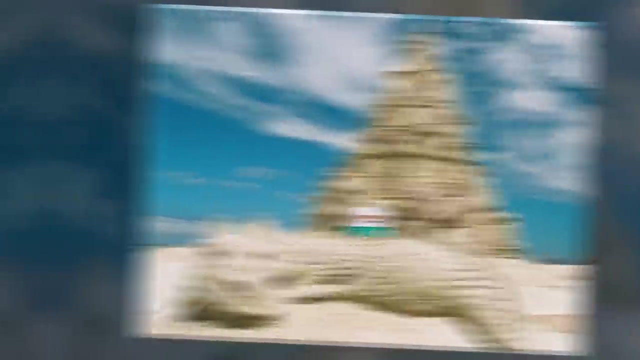 here. I can't tell whether that's just the weather or whether the photo has been through a filter. Either way, the castles are pretty cool. Castle more than makes up for the lack of sunshine. 6. Dragon Sandcastle. Alright, let's take things back to Harry Potter for a second. Did you know that the Hogwarts motto 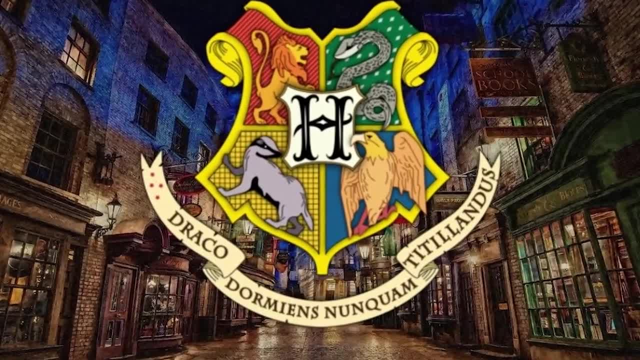 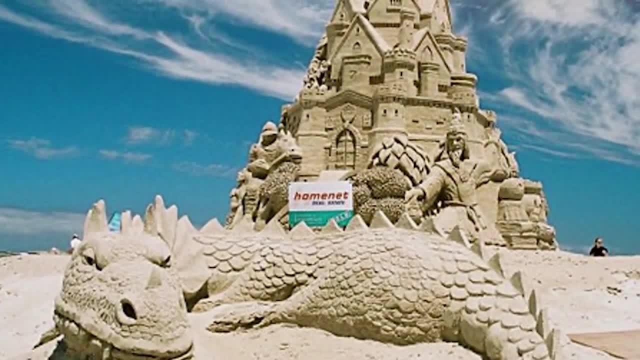 Draco Dormens Nunquam Titillandus. translates from Latin into English as Never Tickle a Sleeping Dragon. This impressive sand dragon isn't quite asleep, but he's not far off either. Still, you're gonna have to get rounded if you want to pay a visit to this stunning sandcastle. 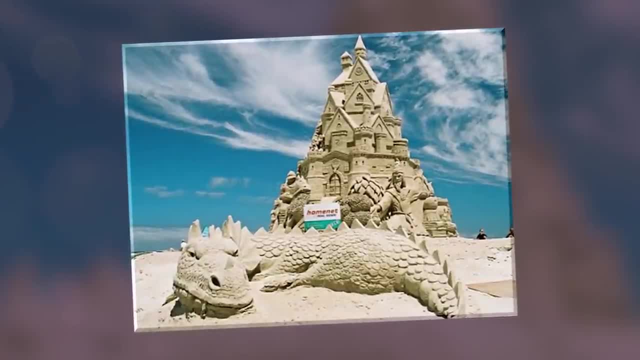 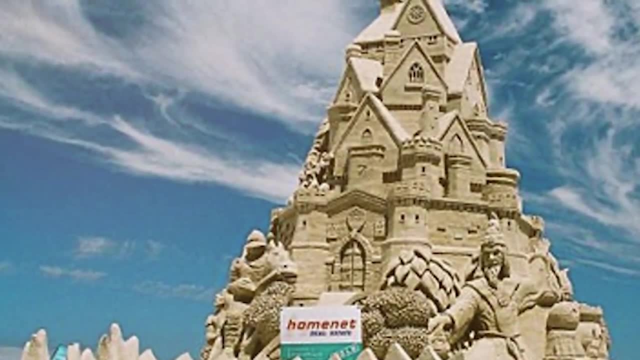 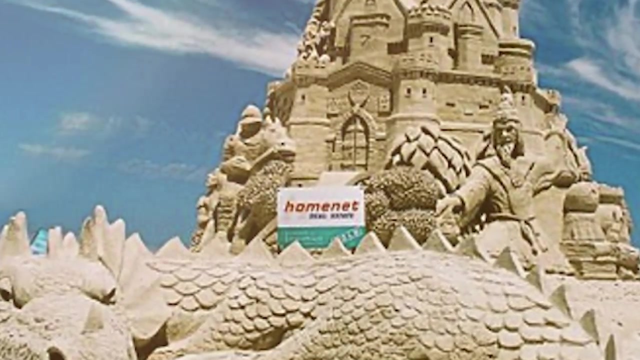 design. 5. Illuminated Sandcastle. This is another one where the attention to detail is very impressive, and I imagine that the bushes were particularly difficult to get right. It's just a shame that the effect is diminished by the advert for HomeNet. Still, it doesn't spoil the overall effect completely and the only thing that 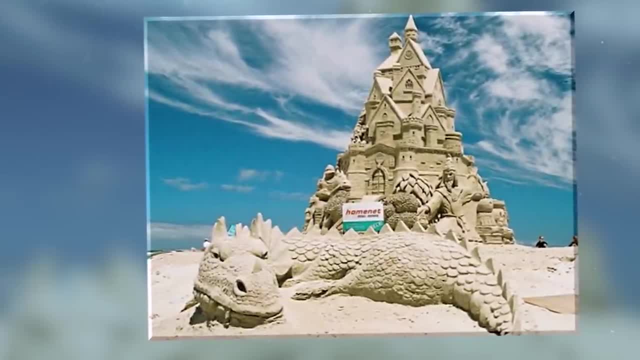 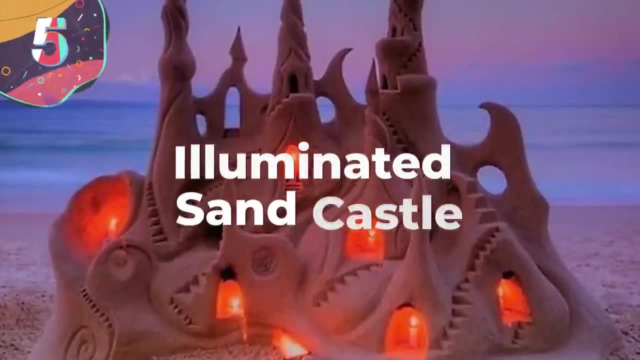 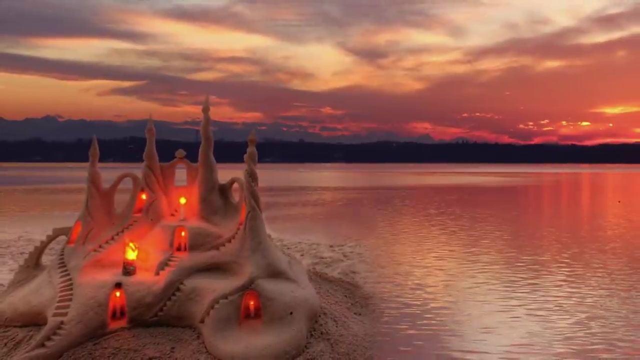 I can really complain about is that the photos aren't of a higher resolution. I'd love to be able to zoom in and take a closer look at this thing. 5. Illuminated Sandcastle. I mean, you only need to take one look at this to see how cool it is. For a start, there's the sandcastle. 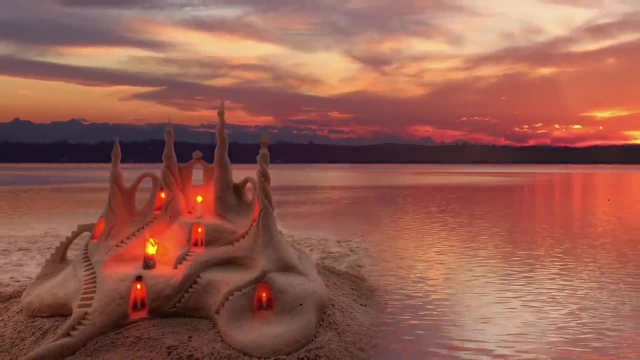 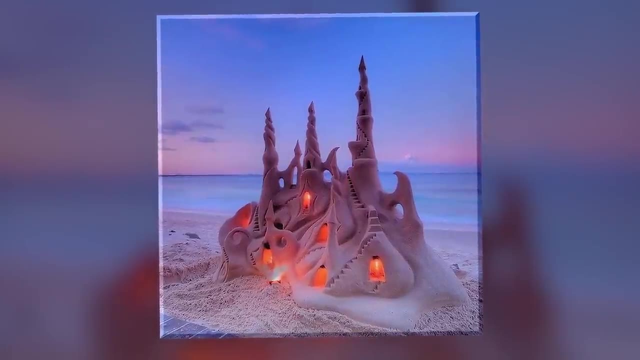 itself, which is much more fluid than the other designs and makes use of a bunch of curving walls. That alone makes it an interesting challenge for its designer, because it must have been hard to build out the structure without it collapsing. The whole aesthetic is then taken. 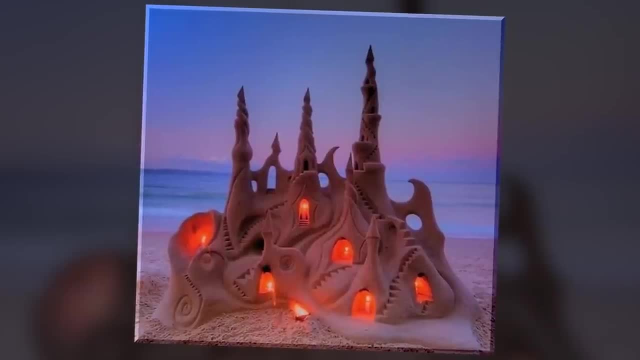 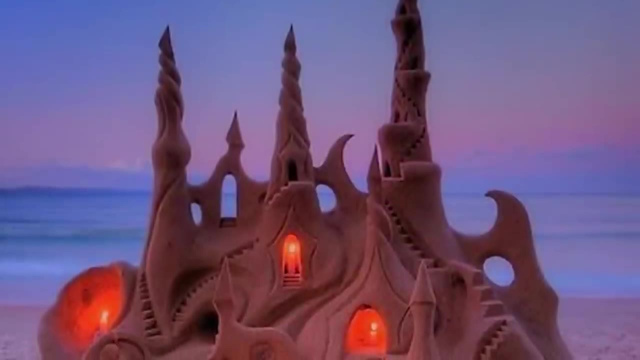 to the next level thanks to its illumination, which takes on the format of a half dozen tiny candles. During the daytime. that would be pointless, but you can see from this photo how effective it becomes when it's dusk. The result is one of the more interesting designs on this list. 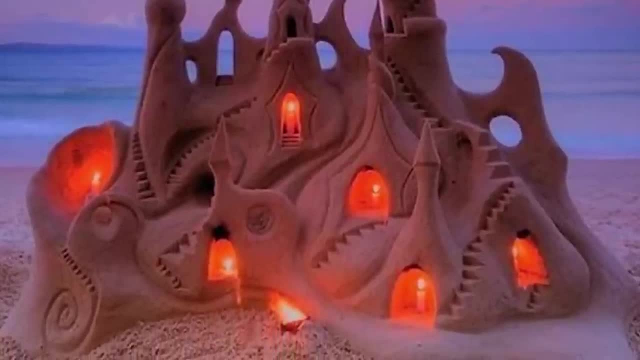 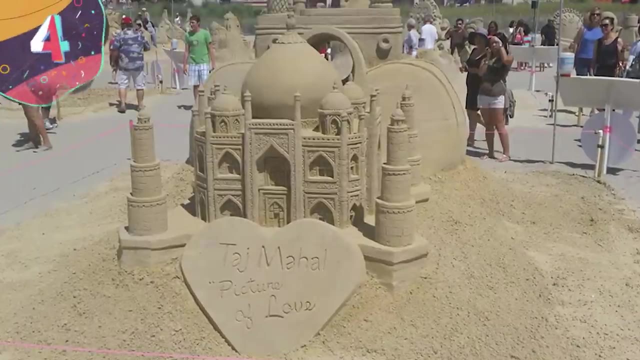 and one that challenges our preconceived ideas of what a sandcastle has to look like. Kudos to its creator, whoever that might be. 4. Taj Mahal Sandcastle. I mentioned the Taj Mahal earlier, but I couldn't call that a Taj Mahal sandcastle when there's 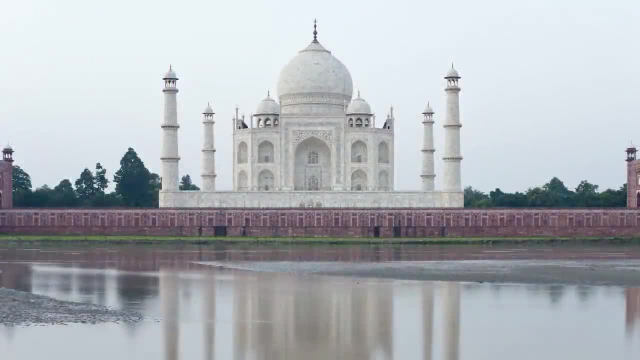 this one on our list, which is a recreation of the iconic palace, as opposed to just a design that's inspired by it. The Taj Mahal is a very interesting design and it's a great way to start off the day 4. Taj Mahal Sandcastle. 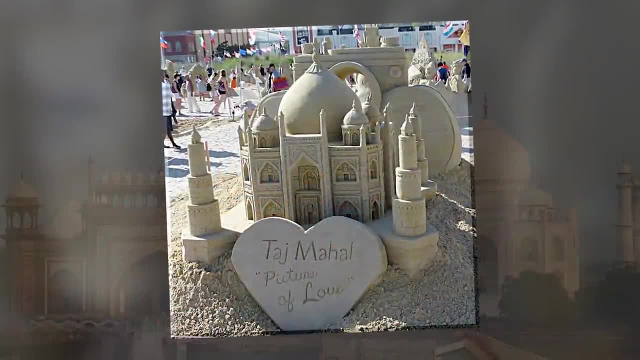 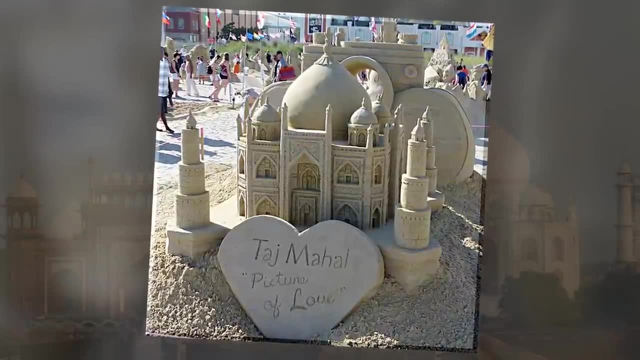 The crazy thing here is that it's actually one of the easier designs to pull off, at least on this list. That's because they had a visual of the actual Taj Mahal to work from and some of the elements, like the rounded tops, are relatively easy to build. 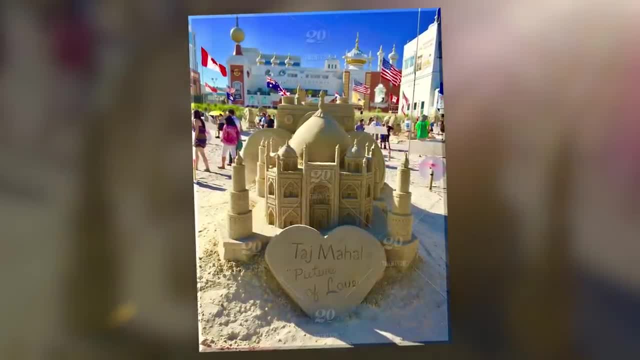 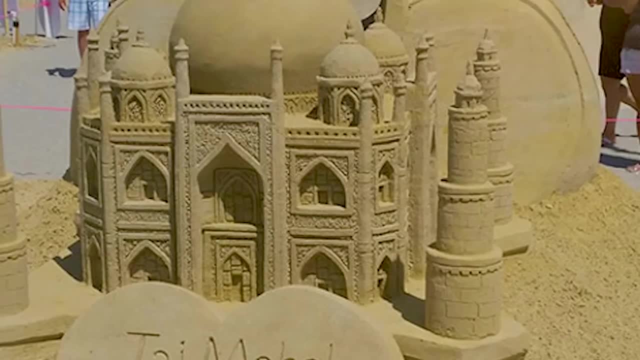 Still, there's a hell of a lot of attention to detail here, at least where it matters. It seems also a little strange that they carved out such stunning brickwork and windows and then just forgot to use a closing quote mark for the phrase picture of love. All in all, though, it's. 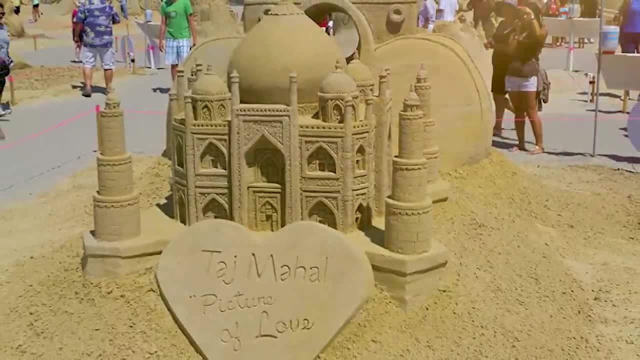 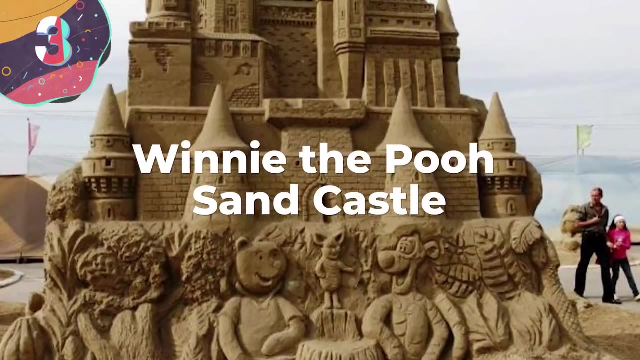 pretty clear from just a quick glance that it's a Taj Mahal sandcastle and it's a great design. 3. Winnie the Pooh Sandcastle: If you have young children, then you're going to love this one- Unless they're so Winnie the Pooh. 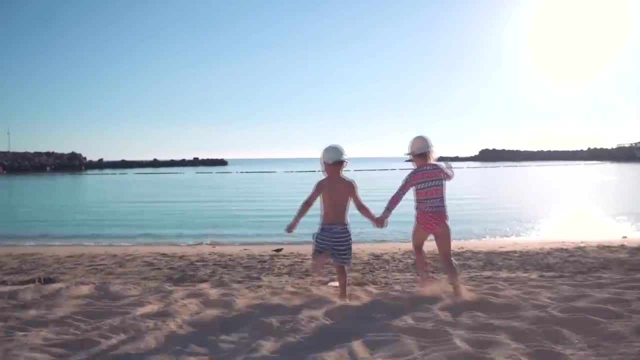 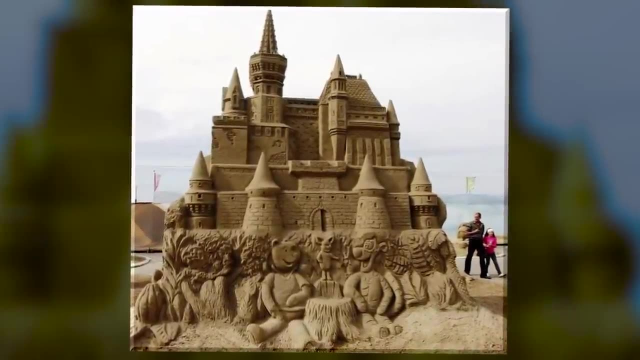 mad that you're sick of it and never want to think about it again. This design is so noteworthy because, as well as being a great example of a well-built sandcastle, it also depicts Pooh, Tigger and Piglet, three of the most well-known and well-loved characters from that series. 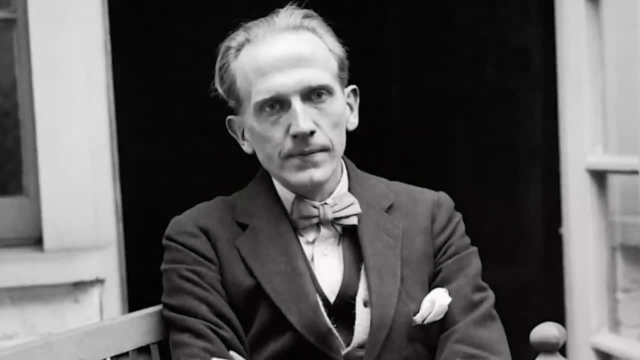 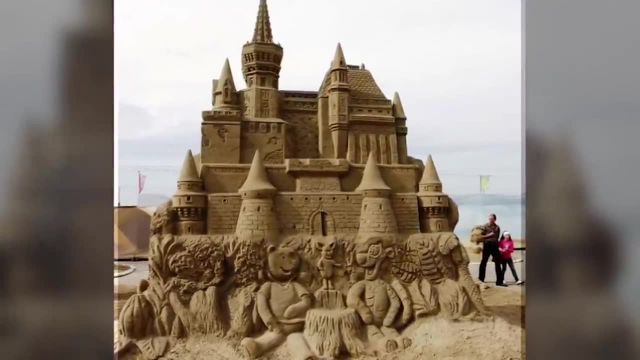 which was created by children's author AA Milne. One of the cool things about this one is that the photo that we can see shows people walking past it from behind, and that can help us get a little perspective. It's not clear just how. 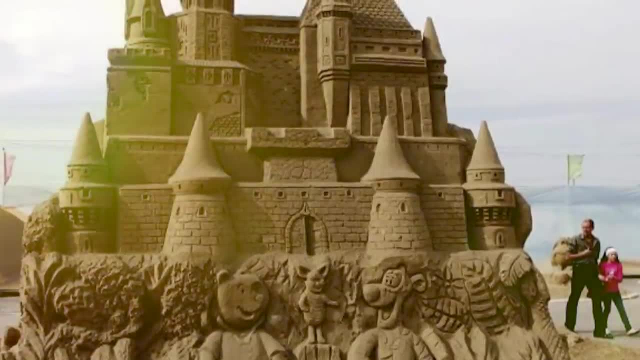 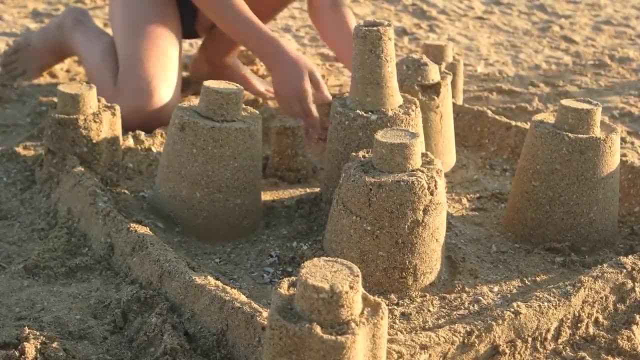 big this sandcastle is, but I certainly can tell it's one of the biggest on this list. Of course, there's also the fact that the sandcastles are intrinsically linked to childhood, and so we love the idea of a design that incorporates some of the most beloved. 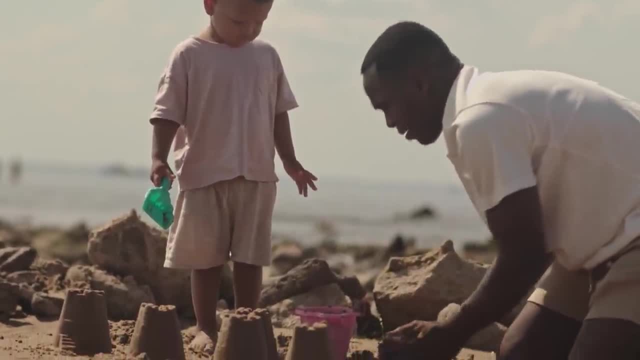 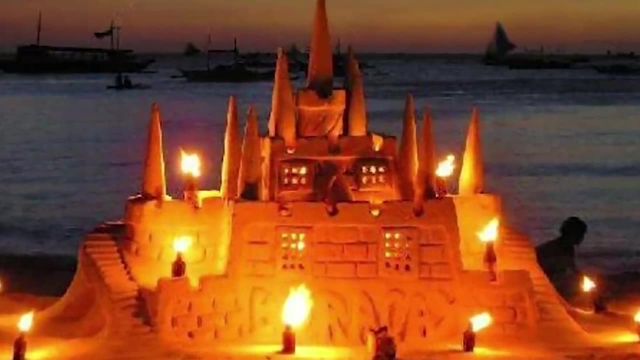 characters in children's books and TV. 2. Torch-Lit Sandcastle- Alright, this is the second sandcastle on our list to be lit up with artificial light, but while the first one just uses candles, this one takes things a step further by using torches. 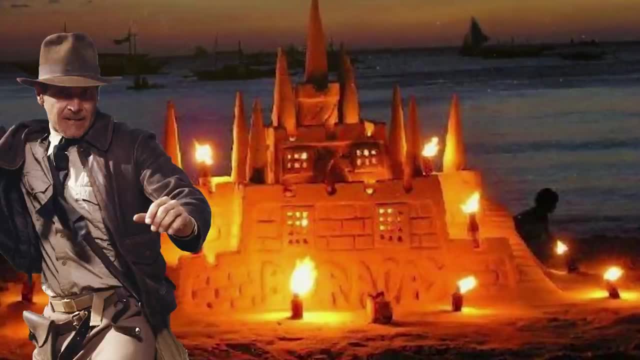 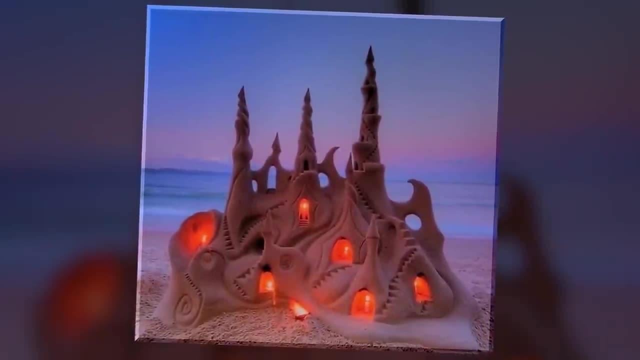 You can almost imagine Indiana Jones grabbing one of them before heading into some long-forgotten temple. Honestly, I have to say that, design-wise, the illuminated sandcastle at number 5 is a little more impressive, though they're both great castles, But when it comes to the overall effect, it's hard to top this one. Not too much is known about who built this one, but the sandcastle is one of the most well-known and well-known castles in the world and it's one of the most well-known castles in the world. Not too much is known about who built this one, but when it comes to the overall, effect. it's one of the most well-known castles in the world. Not too much is known about who built this one, but the sandcastle is one of the most well-known castles in the world. Not too much is known about who built this one, but the sandcastle is one of the most well-known castles in the world. 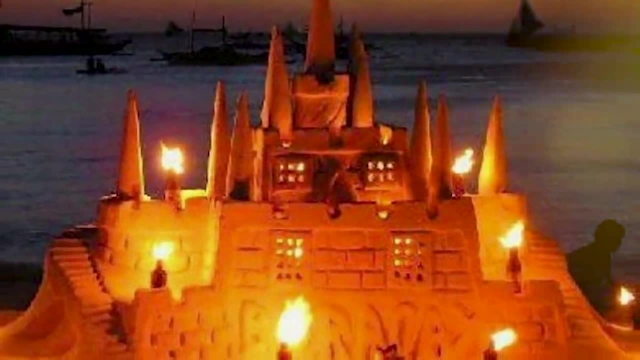 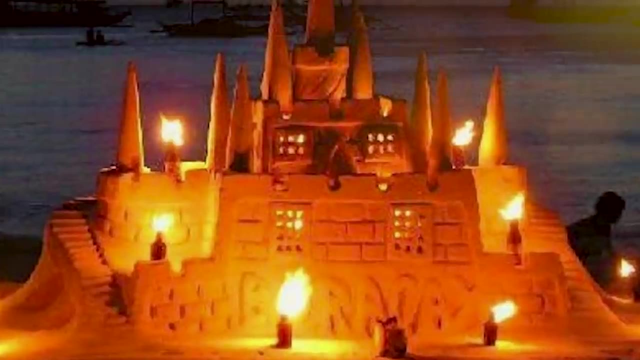 But that's pretty standard for a list like this. I love the conical towers and I'm really impressed by the windows, which are fairly rudimentary in design but look amazing thanks to the interior torches that spill light through them. Overall, you're unlikely to find a cooler-looking illuminated sandcastle. 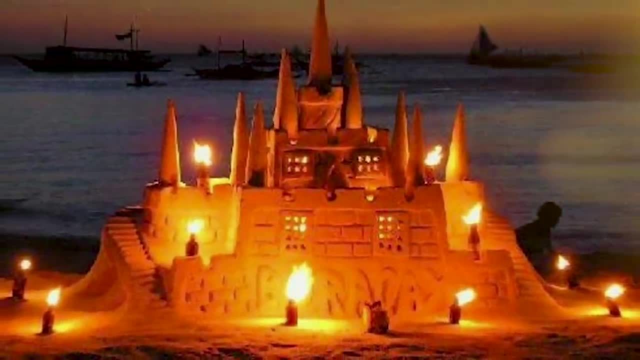 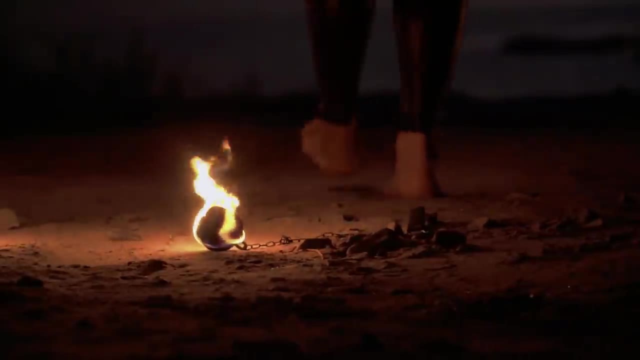 and it's surprisingly difficult to build interior torches into the design. Not only do you need to light them and place them before you finish building, but also you need to make sure that they have access to enough oxygen to keep on burning. Number 1. The World's Tallest Sandcastle.